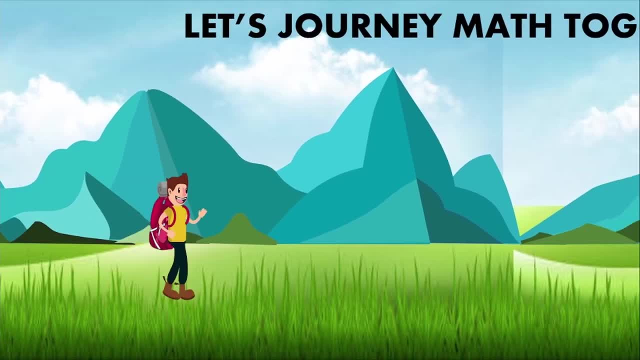 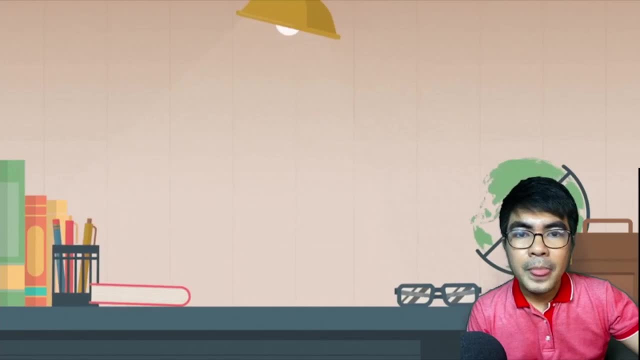 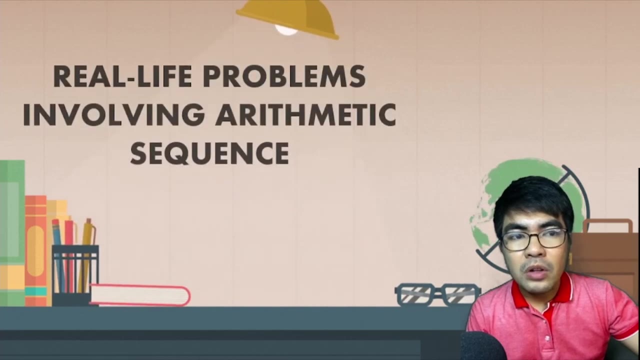 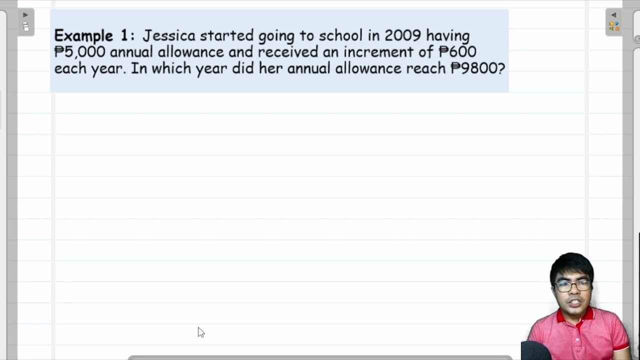 Hi, in this video, you will learn how to apply the concept of arithmetic sequence in solving real life problems. So for our first example, we have: Jessica started going to school in 2009, having 5,000 pesos annual allowance and received an increment of 600 pesos each year, In which year 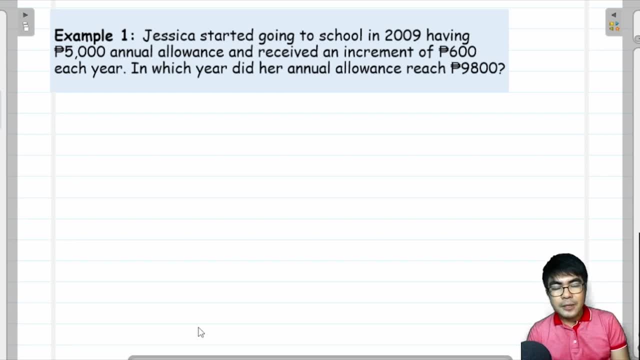 did her annual allowance reach 9,800 pesos? For us to answer this problem, let's be familiar with some of the terms here. Terms are increment, meaning an increase, and annual means yearly. So for us to know the year wherein Jessica reached an allowance of 9,800, let's take note that she 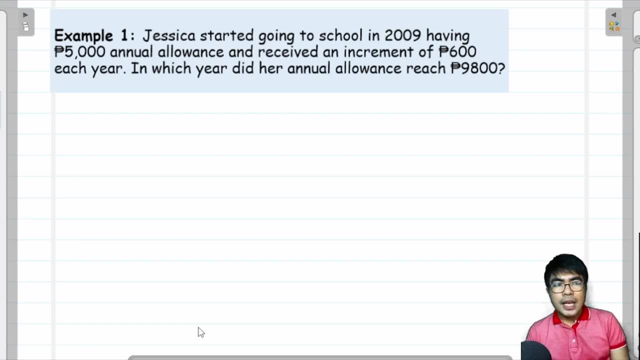 started schooling in year 2009 and that could be considered as the first year, and an increase of 600 pesos each year. So that means to say the following year would have 5,600 right, and every time as year goes by there is an increase of 600 pesos. So the number 600 pesos would definitely 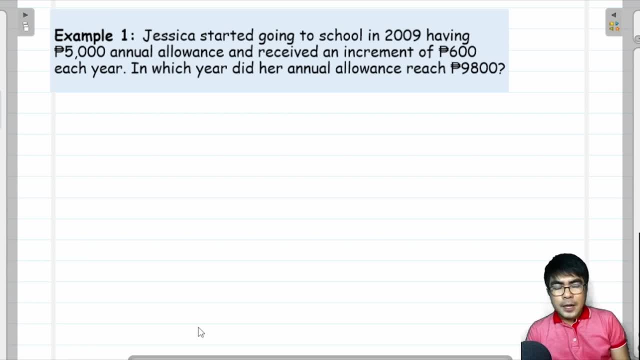 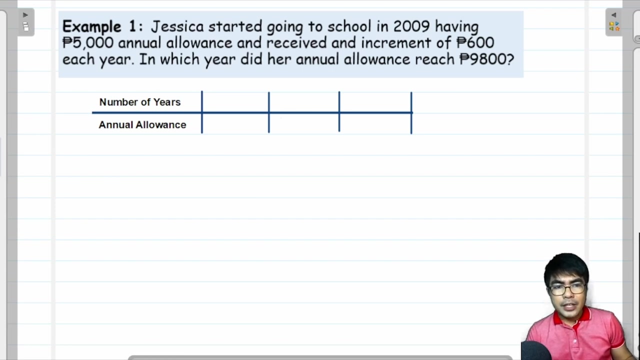 be considered as the common difference, and with that we can treat this problem as an arithmetic sequence, since there is a fixed common difference of the sequence that would be created out of this equation. So for our second example, let's take note that she will make a table of values wherein 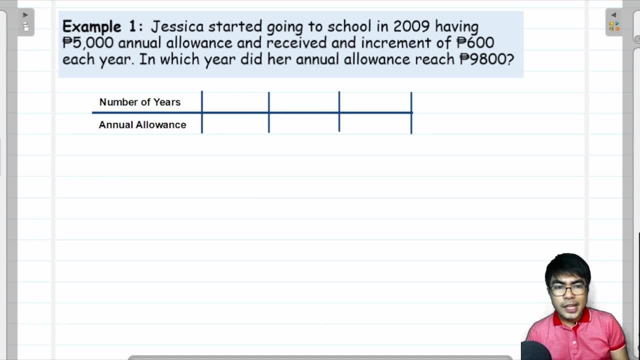 the variables are the number of years. Let's take that number of years as the variable n, and the other variable is her annual allowance. So for the first year in year 2009, Jessica had 5,000 pesos allowance, And on the second year, which is in year 2010, she will get 5,000 pesos allowance. 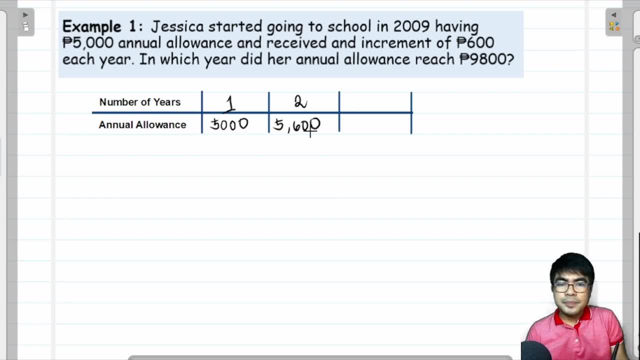 So she will get 5,600 right, and then you add again 600 plus 600 until you reach 9,800. but that would be tedious. So this another alternative method to reach 9,800, apart from adding in 600 every time, is by applying the formula. We know that nine thousand eight hundred is. 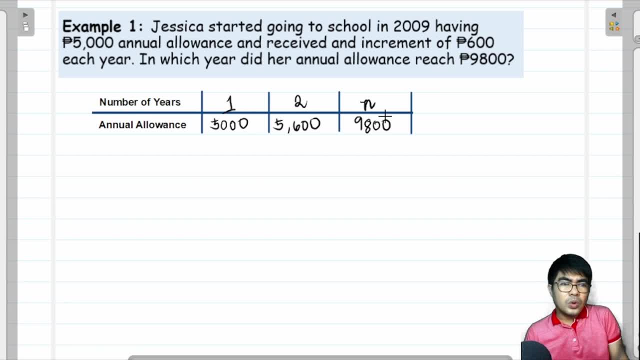 our goal and we still don't know the end there. meaning the number of years. And let's be guided with the formula: a sub n equals to the first term plus the common difference times n minus one. By substitution, we know that a sub n is 9,800. 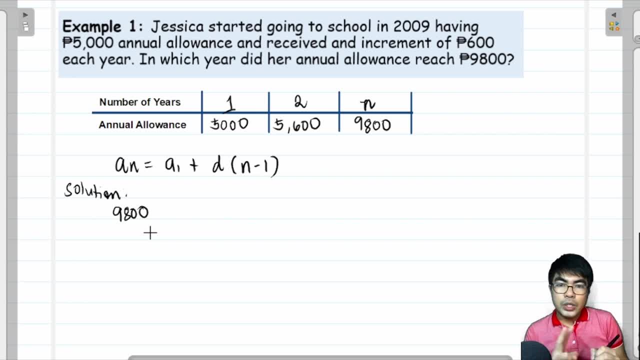 It's like similar to the case number two in the previous video, wherein we are looking for n here. The first term is obviously 5,000 pesos plus the common difference of 600.. Copy: n minus one. so we're looking for n here, So we know that we can cancel 5,000 and. 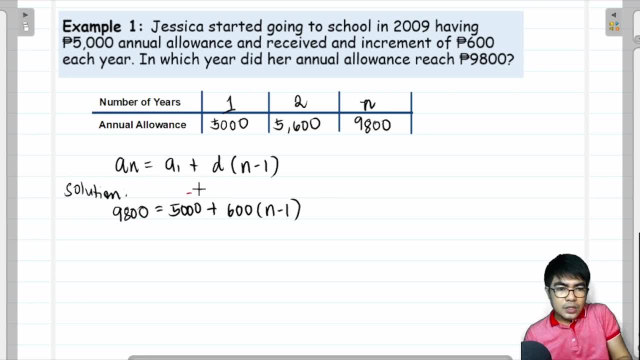 9,800 because they are constant. So to eliminate 5,000, so we add both side by the inverse of 5000, which is negative 5,000, So this becomes 0, and 9,800 minus 5,000 is 4,800 equals. 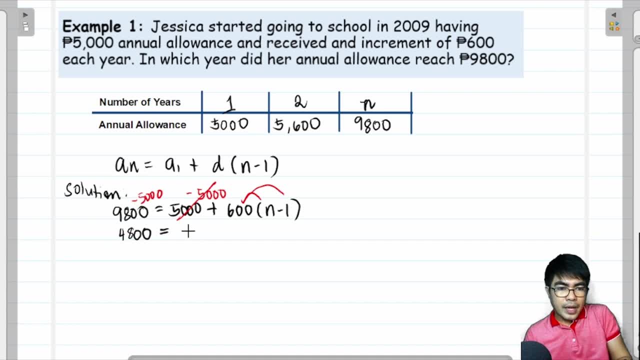 distribute 600 to n minus 1 by multiplying it, so this is 600n minus 600, since it's 600 can be added to 4800, since they are constant. so we will add both sides by the inverse of negative 600, which is positive 600, and then the sum of 4800 and 600 is 5400, equals what's left. 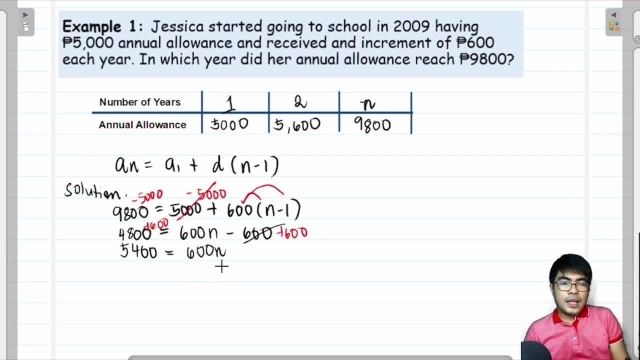 here is 600 n, and then to isolate n we divide both side by 600 and then cancel this. 2054 divide 6 is 9, therefore our n is 9 years. so after 9 years Jessica will get an allowance of nine thousand eight hundred. since the question here is in which year? so the year she started is 2009, so count of nine times from 2009. so since 2009 count as one, so we will just add 2009 by 8, not 9, because 2009 already. 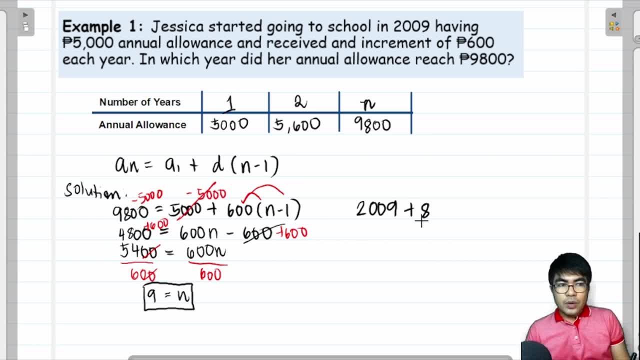 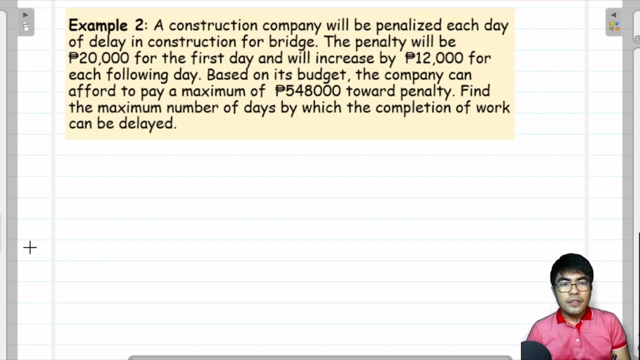 count as one, so by nine years Jessica would have 9800, and that year is in year 2017. okay, so that is just how we apply that problem. next problem is a construction company will be penalized each day of delay in construction for bridge. the penalty will be twenty thousand pesos for the first. 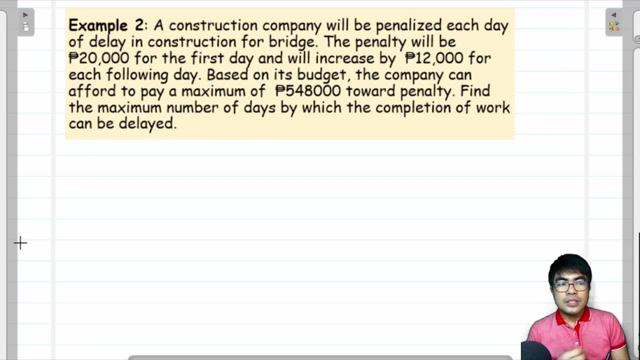 day and will increase by twelve thousand pesos for each following day. based on its budget, the company can afford to pay a maximum of five hundred forty eight thousand pesos toward penalty find the maximum number of days by which the completion of work can be delayed. so the approach here will be: 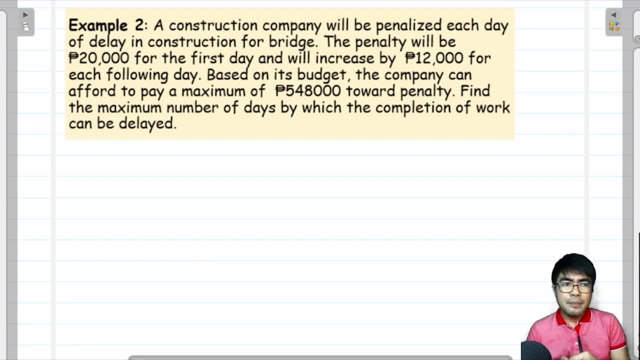 somewhat similar to what we had in the first example. we will illustrate that, or we'll draw a table of values where in the first variable is the number of days, since the penalty for the first day is twenty thousand and there will be an increase of twelve thousand pesos each day, so we can presume that the first day is twenty thousand. okay, it's. 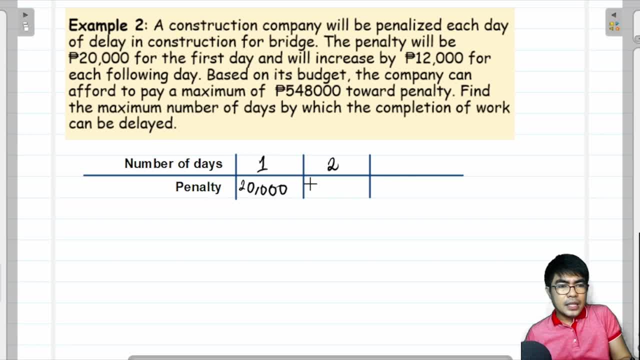 twenty thousand and on the second day, expected that it will be thirty two thousand. okay, what is the maximum number of days by which the completion of work can be delayed, which is: the company can only afford to pay a maximum of 548. this is the Max, this is their budget. so what is the equivalent days for? 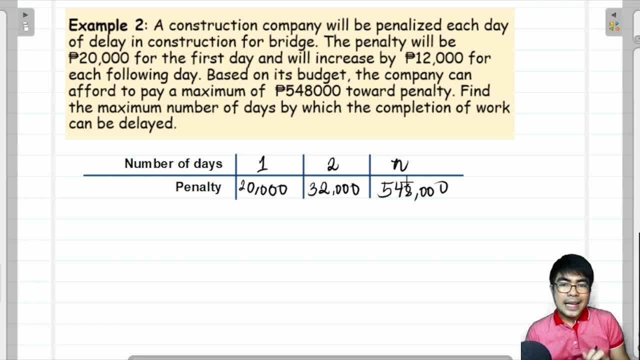 five hundred forty eight thousand pesos, so we will assume that as n, so using the same formula. since the problem is about arithmetic sequence, we will still use this formula: first term plus common difference times n minus one, ours, our a sub n, here is five hundred forty eight thousand pesos. 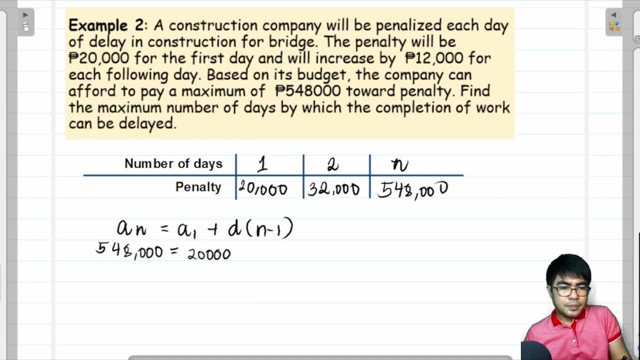 and the first term is twenty thousand plus the common difference of twelve thousand pesos times n minus one. so we can add twenty thousand both side by its inverse, and the inverse is negative. twenty thousand subtract both side, and then the difference on the left-hand side is five and minus one, and after the up your mark then. 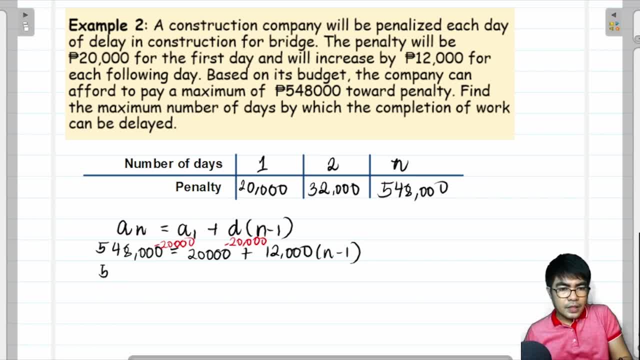 the difference is negative. twenty thousand times n minus one plus one, and we areauf the inverse is an. 528,000 pesos equals 12,000. distribute it to n minus 1 by multiplying, so it's 12,000, n minus 12,000. so add again both side by the inverse of negative 12,000, that's positive 12,000. 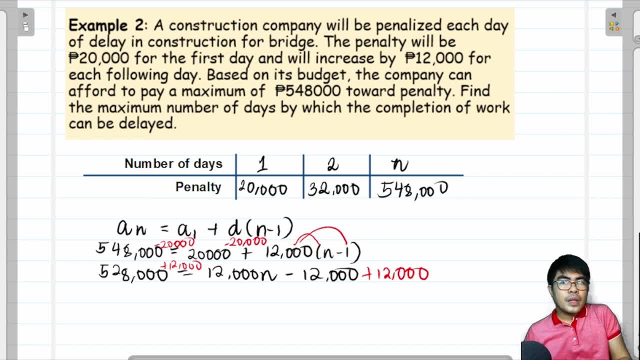 and then this will be zero. on the right hand side you only have 12,000 n and then 528 to, and then 528,000 plus 12,000 is 540,000. so we will divide both side by 12,000 to isolate n. 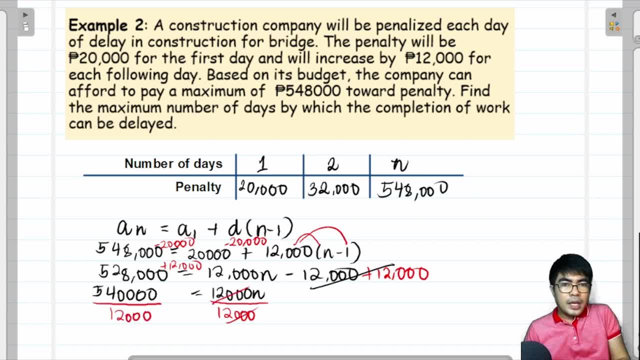 and then this will be n. the right hand side is n, and then we can eliminate this three zero and then 540 divide 12 can use a calculator here class. so we have 45, so the number of days is 45. so you can conclude here that the number or the maximum number of days by which the completion of